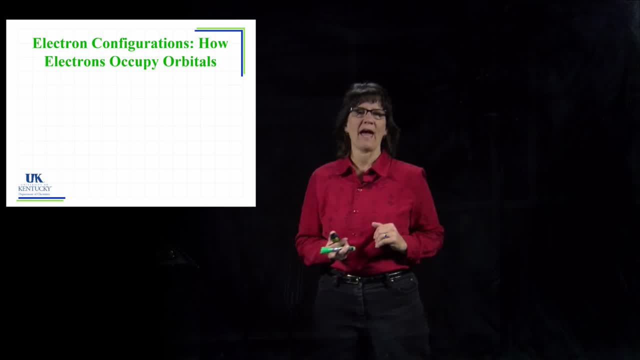 just how those electrons are occupying the orbitals within an atom. So we learned what orbitals exist. We learned about orbitals. we learned how they're grouped together in sub shells. we learned how those sub shells are grouped together into principal shells. those shells and principal shells and orbitals get occupied by 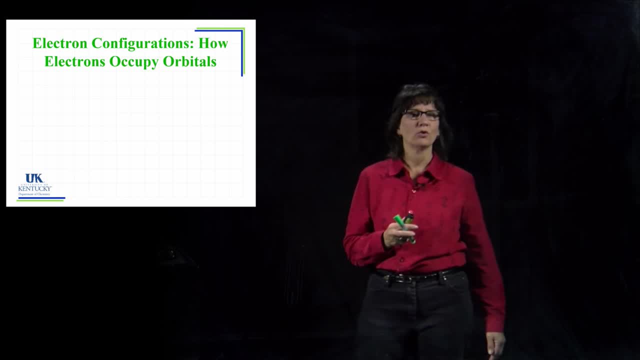 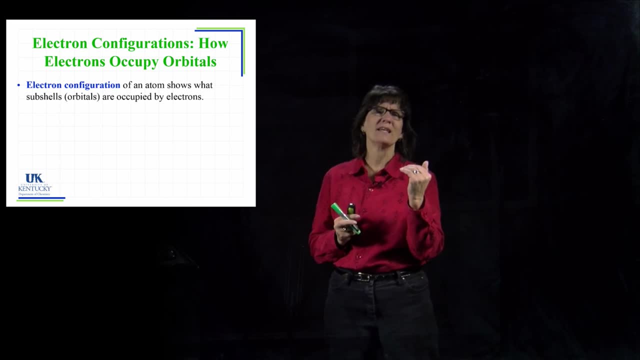 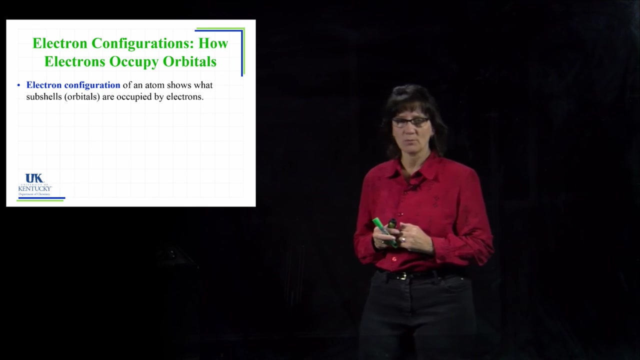 electrons, And so the electron configuration is how those orbitals are occupied. So it shows when we do an electron configuration we're basically only doing it to the shell and sub shells level. we'll tell what the sub shell is and how many electrons are in that sub shell. 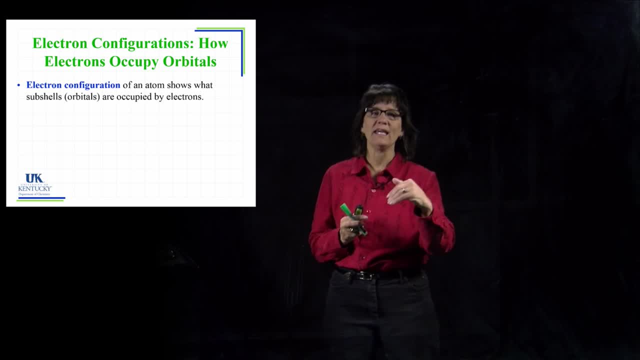 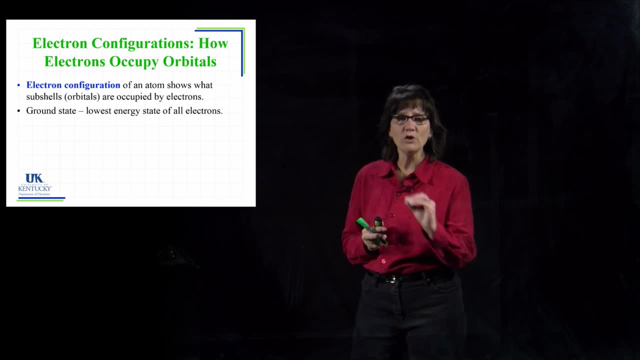 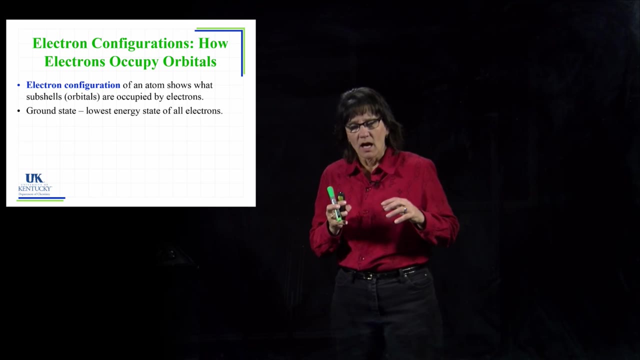 By our knowledge about the orbitals and how many orbitals are in each sub shell, we can also know where they are in the orbitals themselves. When we do an electron configuration, we will always do it for the ground state. What does that mean? We're going to put electrons in and making sure 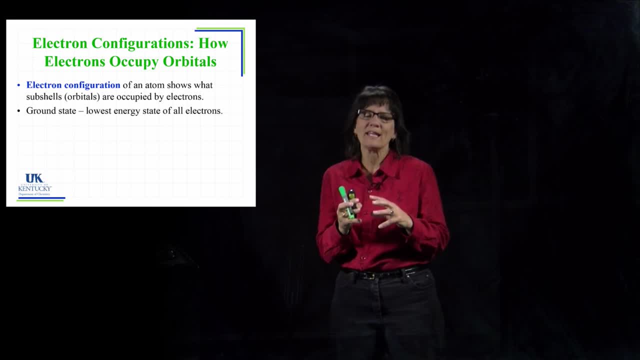 that the lowest energy orbitals are filled first, and then, when that gets filled up, we'll go out to the next higher one and on. And we'll always, when we're asking for an electron, always be asking for the ground state, because you can take electrons and they. 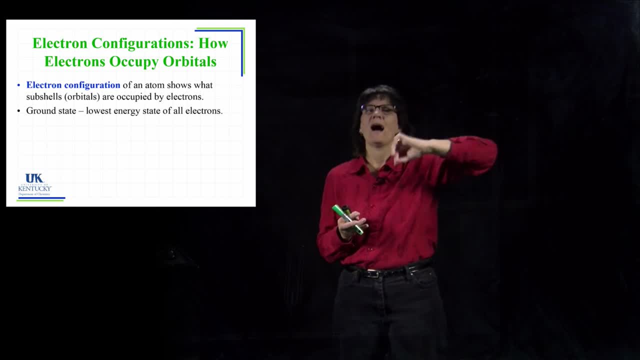 can be up somewhere up in a higher orbital, somewhere a higher, in a higher s and p value, somewhere higher and farther away, and it is an electron configuration but it's not where they're all ground state and that it helps us. just have a common language across all of the atoms. okay, so our first one. first, 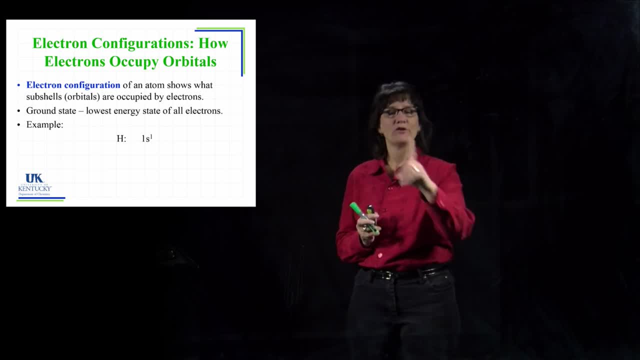 example, would be the simplest atom. it is hydrogen. hydrogen only has one electron, and so when we place that electron into its orbital it's going to be the lowest end, because we know that the smaller the end, the closer it is to the nucleus, and so that's an n equals one. we know that there's only one sub. 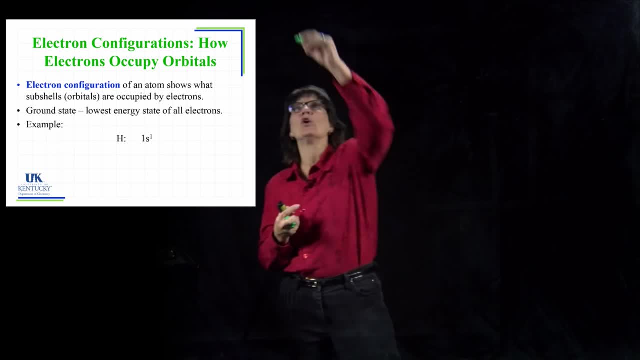 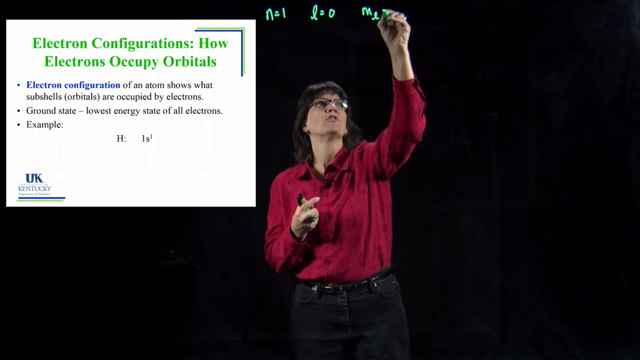 shell in the n equals one, and we did this last time. we learned that when n is equal to 1, L is equal to 0 and M Sabel is from a negative 0 up to positive 0, only that. so this tells me in the 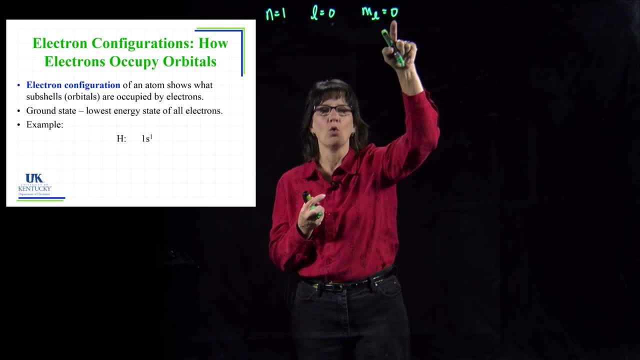 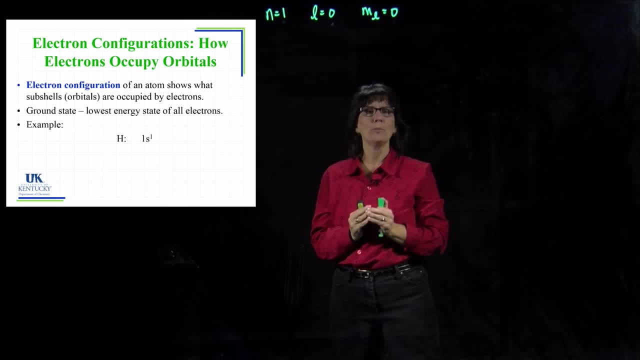 first shell, there's an s sub shell and there's only one orbital in there. so that is the closest to the nucleus, that's going to be the lowest energy and if we're going to put the one electron that hydrogen has into that orbital, that's how we denote it. we denote it with the one telling me that in we 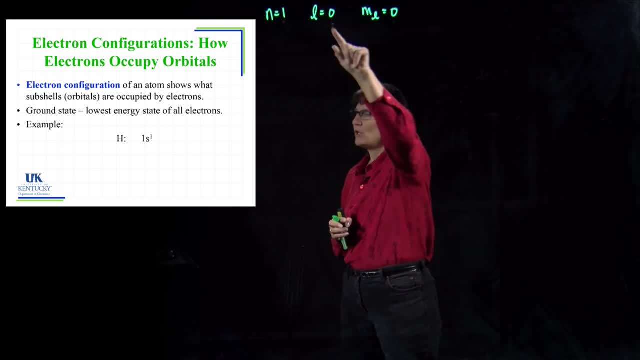 denote it with the s telling me it's in that sub shell. and then we do a superscript of a, one that tells me we have one electron in that sub shell, all right, so one s is the name of the sub shell and that one right there tells me: 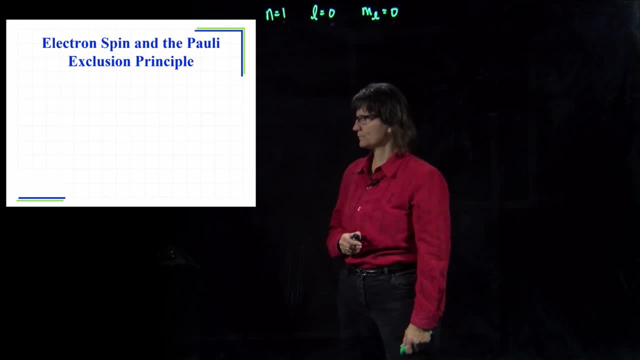 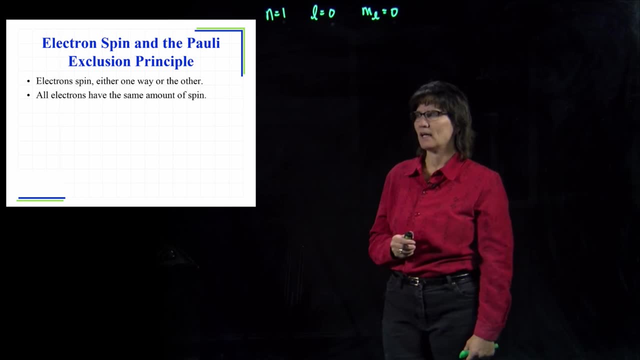 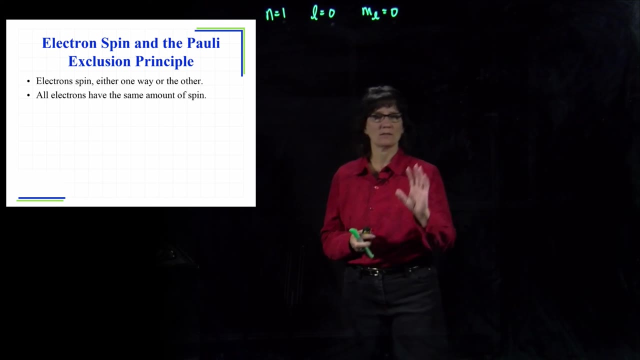 I have one electron in that sub shell, so the next quantum number we have to deal with is the Pauli. what we're going to talk about the Pauli exclusion principle, and we're talking about the spin. so we know that electrons. you didn't know this. 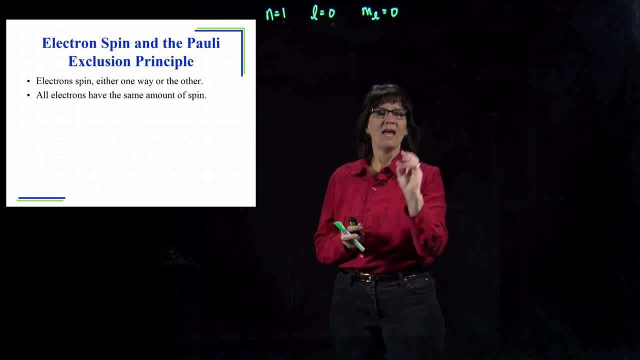 until now, or maybe you did. but electrons spin. okay, they have a spin to it. it gives them a little, makes them behave like a little magnet. okay, and they have an option. they can either spin one way or they can spin the other way, and that's it okay. so 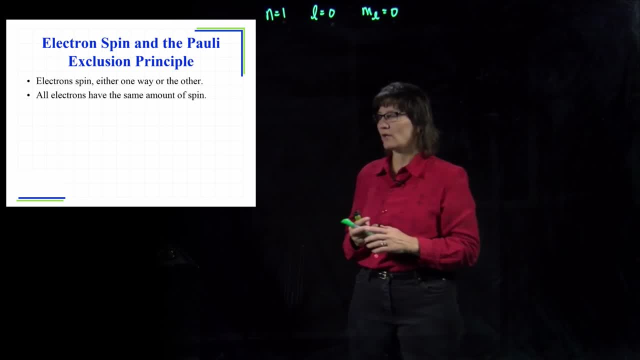 there's two directions to their spin. all electrons are going to have the same amount of spin value- wise- but one will spin in one direction- maybe we'll call it clockwise, and the other one will spin in the other direction- we'll call it counterclockwise. okay now, clockwise and counterclockwise means how are you? 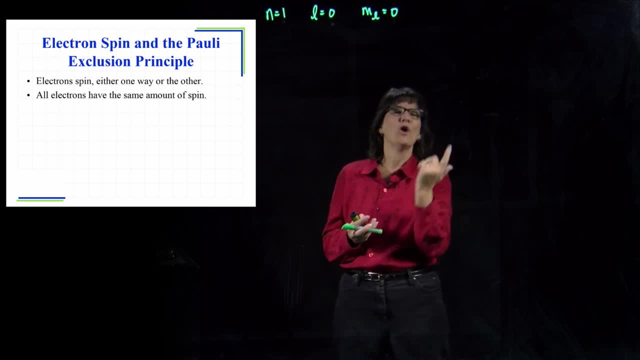 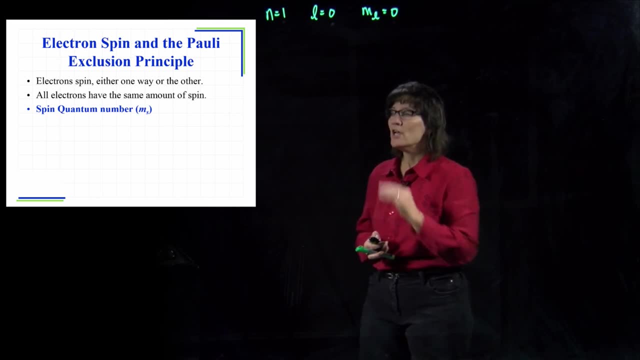 looking? are you looking at from the top down? even from the bottom up? I don't know. but once you call one clockwise, the other one is spinning the other direction. we'll call it counterclockwise, so we'll use that language with it. okay, so our spin. 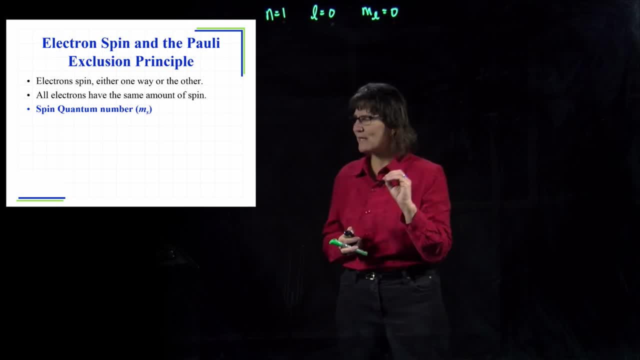 quantum number is abbreviated m sub s, and that spin quantum number, m sub s, is basically giving us a value for that spin. there's only two options. it can either spin plus 1 half or minus 1 half. okay, so if plus 1 half is the one we 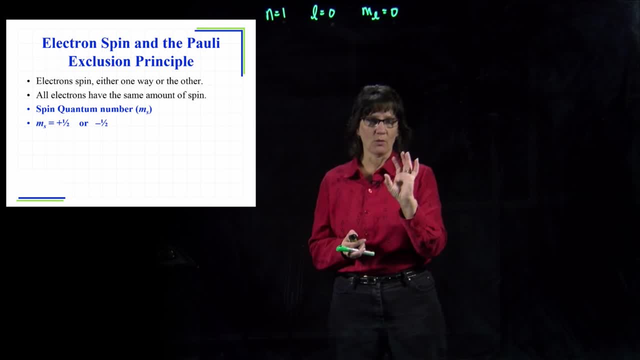 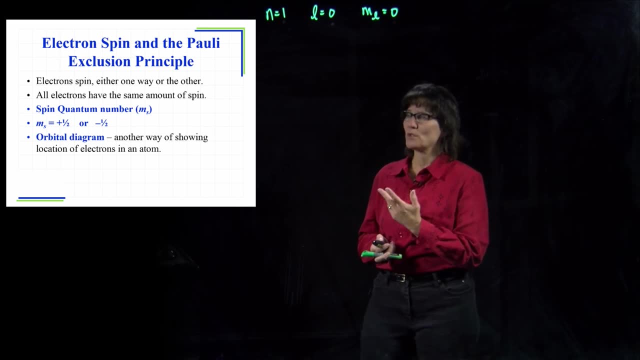 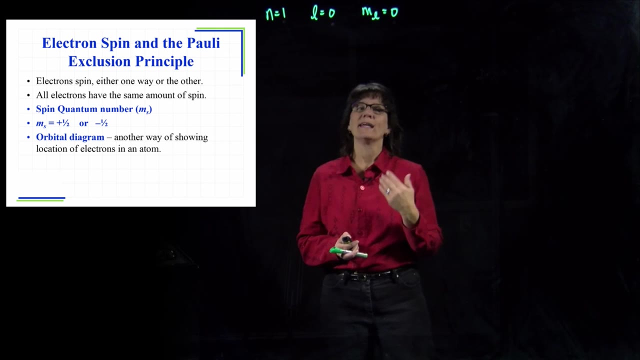 called clockwise, then minus 1 half would have to be counterclockwise. those are the only two options for the spin. now we can, besides doing electron configuration, which we saw before with the 1ays, with a superscript 1, that's an electron configuration we can also give. 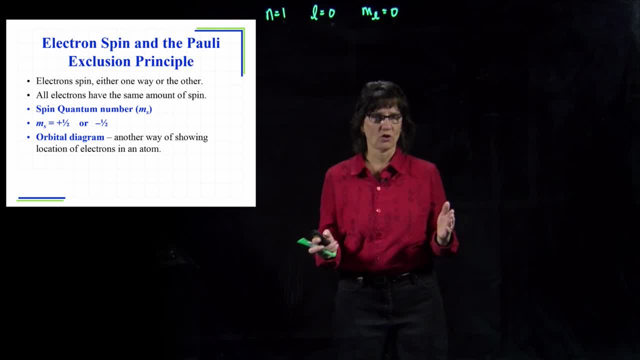 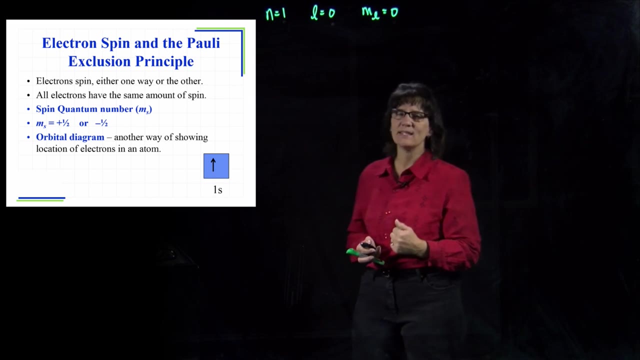 an orbital diagram for its electronic structure. so those are the two ways that we can show where the electrons live. the orbital diagram gives more information than an electron configuration, so it is just another way of showing where the add electrons are in the atom. and this is the orbital diagram of theNA Asians. 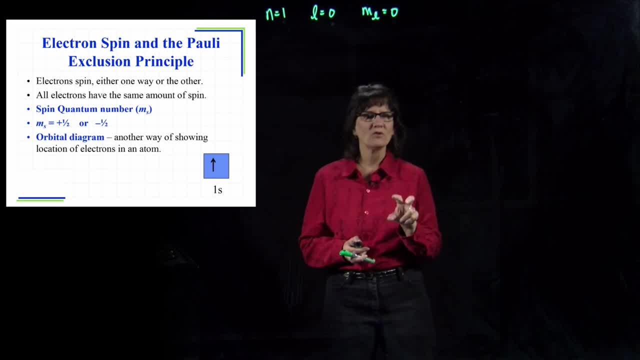 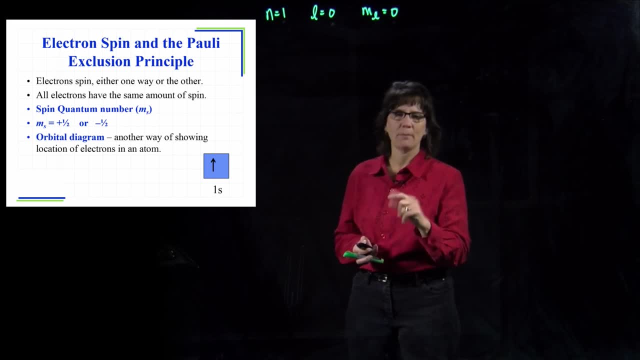 for hydrogen. What is represented here? Well, the box is representing the orbital, which is a 1s orbital. We see that underneath there, And the arrow that's pointing up is representing the spin of the electron. So if the electron is spinning in one direction, we put an arrow pointing up. 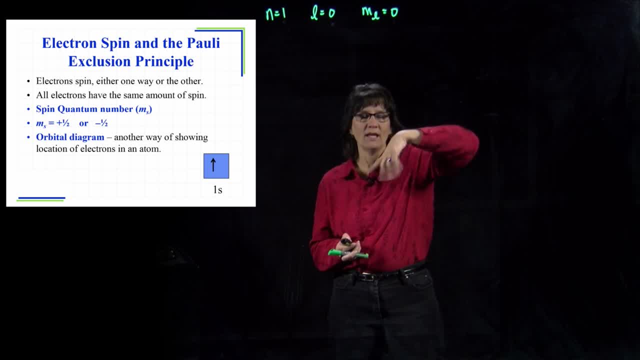 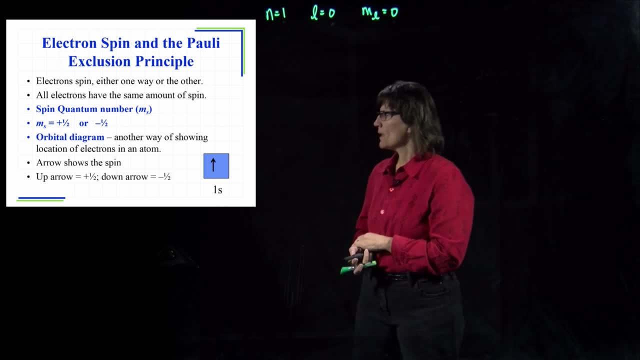 If it's spinning in the opposite direction, we put an arrow pointing down, Now typically. well, I'll get to that in just a minute, okay. So that arrow is just showing the spin of the electron. So I always though this is just my standard way of doing it. 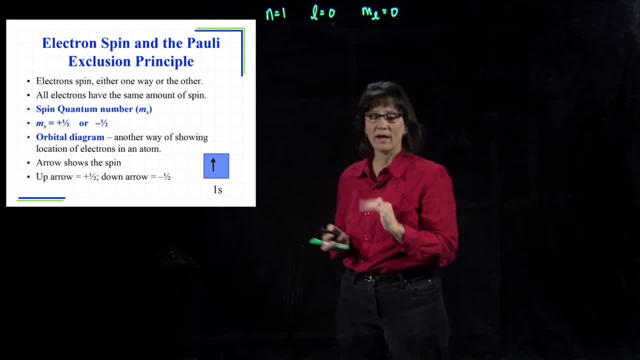 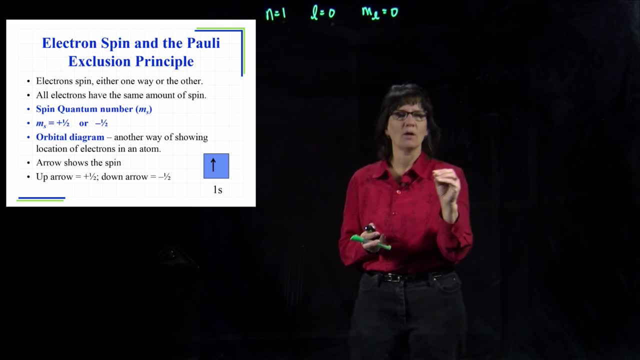 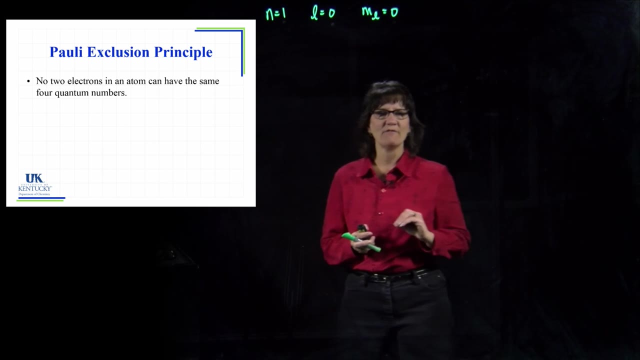 is my up arrow, is my positive one-half spin, And if you have a down arrow, it would be the negative one-half spin. So I'll always use that relationship for the direction of the arrow and the value of n sub s. Now, this is a very, very essential thing that we need to know about electrons. 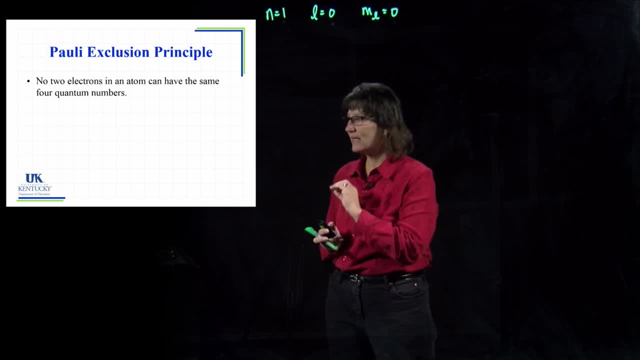 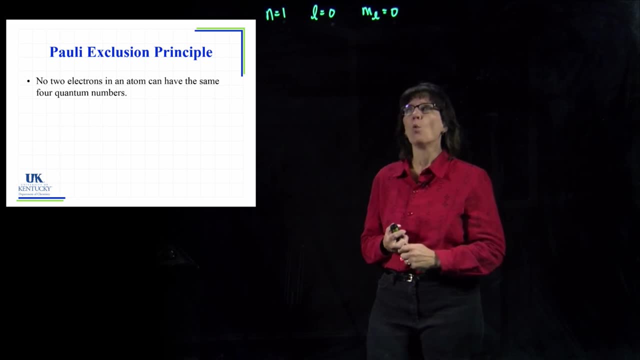 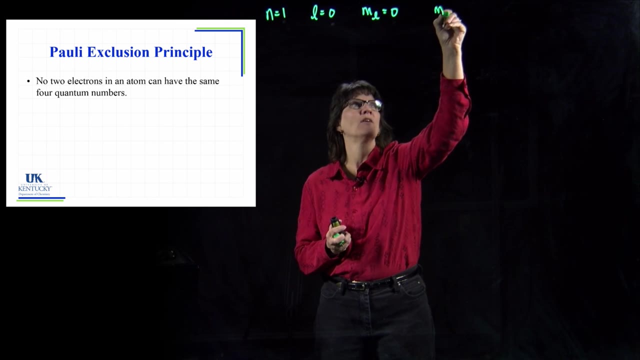 Two electrons in an atom. Sorry, I should say it this way: No two electrons in an atom can have the same four quantum numbers. What are those four quantum numbers? Well, we have the n, we have the l, we have the n sub l and now we have the m sub s. 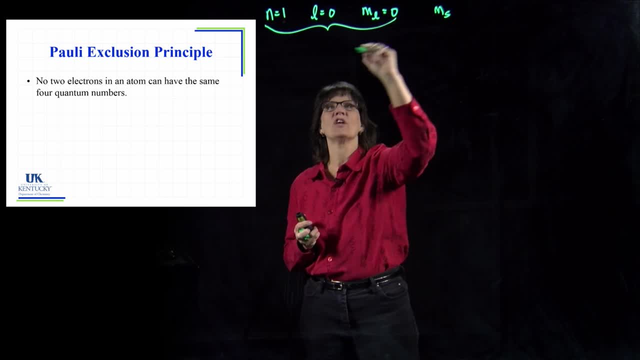 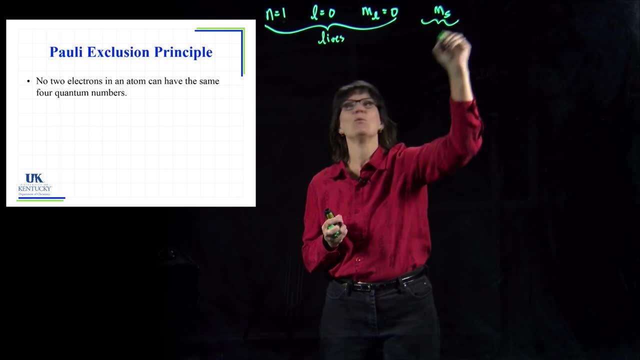 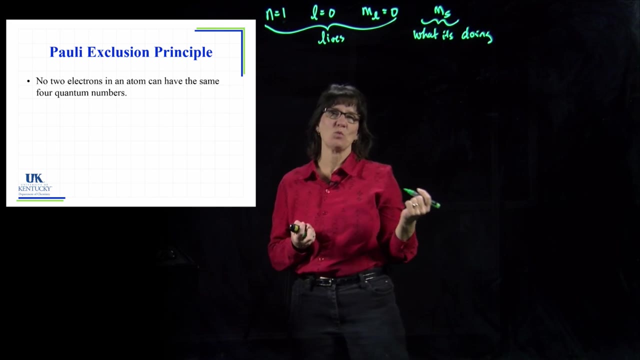 Now, the way I think about these is: these electrons are telling me where the electron exists, okay, Where it lives, I'll call it that. And this is telling me what it's doing. Alright, It's spinning, and it tells me which way it's spinning. 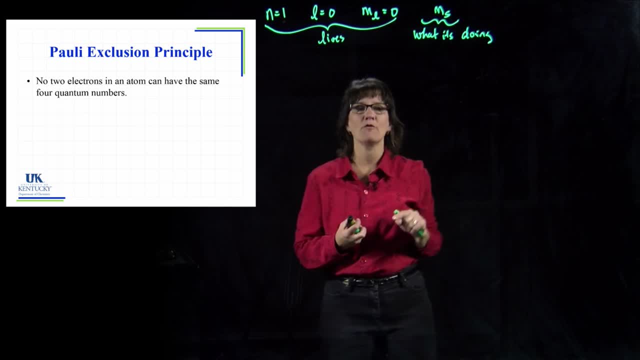 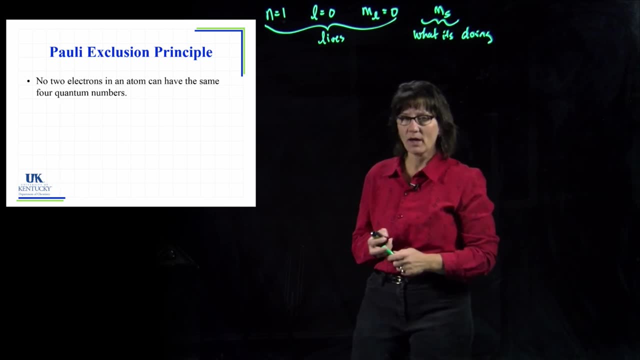 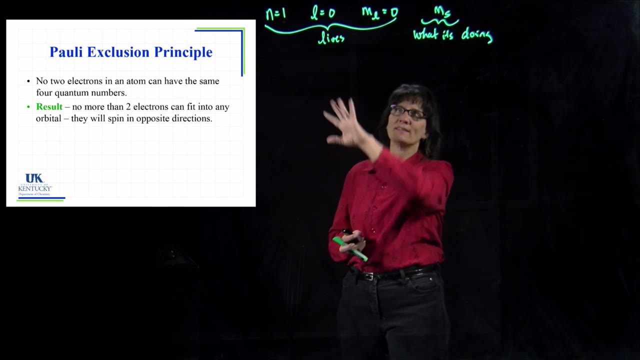 No two electrons can have the exact same four quantum numbers. They can have three that are the same. as long as the fourth one is different, we'll be okay. So what is the result of that? This is the bottom line. So Pauli Exclusion Principle has to deal with the quantum numbers. 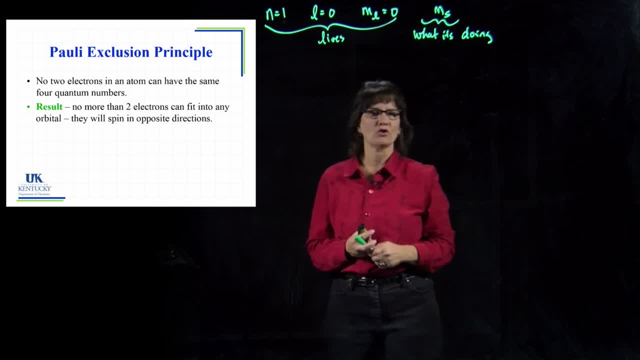 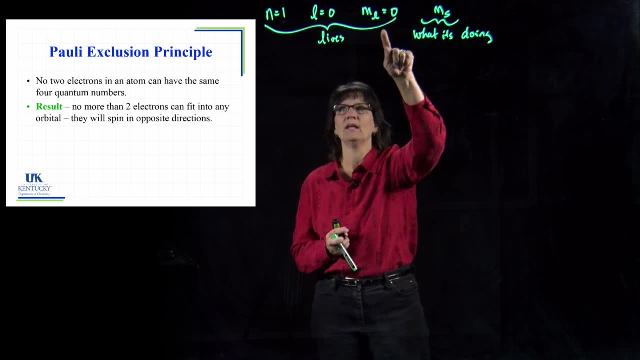 The result of this is that you can have no more than two electrons in any orbital. okay, Because all three of these numbers together define right down to the orbital it lives in. It lives in the first shell, it's in the s subshell, it's in this orbital. 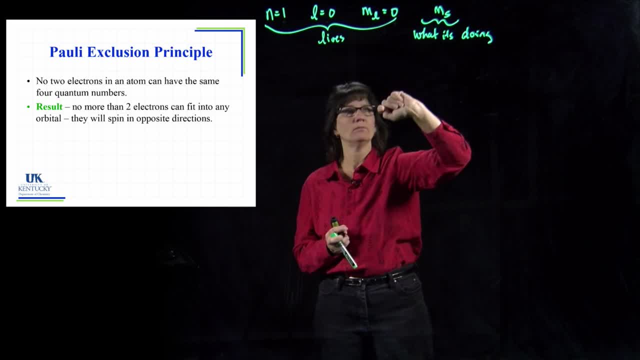 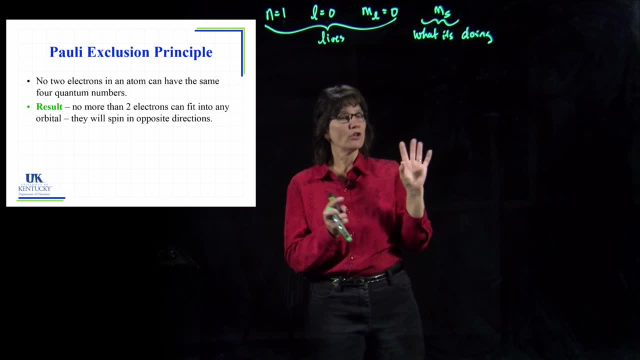 And we can have one electron spinning one direction and we can have one electron spinning the other direction. That gives that m sub s a different value. So as long as you have two electrons spinning in the opposite direction, they can exist in that orbital. 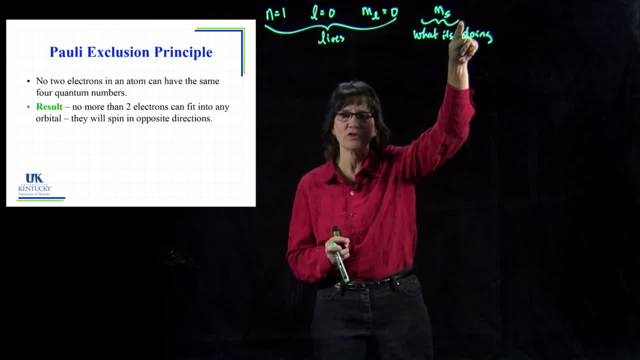 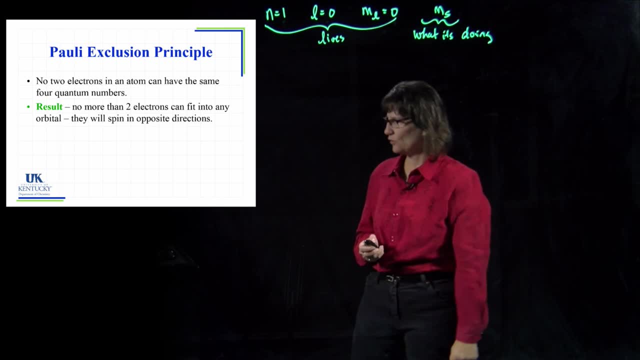 But as soon as you try to put a third one in there, it has to either spin plus one half or it has to spin minus one half, And once you have those values, you can't have a third one with those same values. alright, 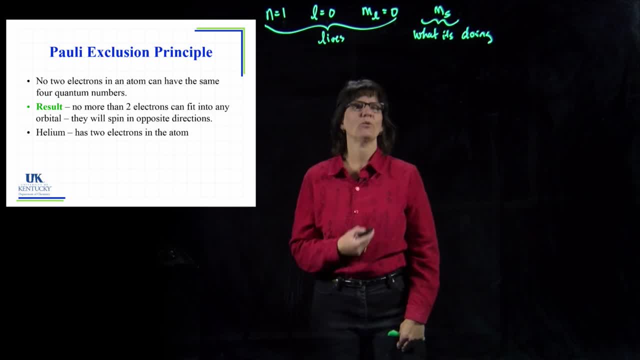 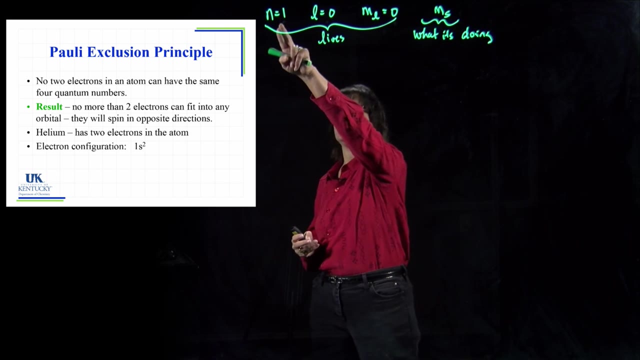 So we can go to the next atom and do the electron configuration and the orbital diagram of helium. Helium is the next element on the periodic table. It has two electrons. okay, So the electron configuration is one s two. Those two electrons are in the one shell, the s subshell. 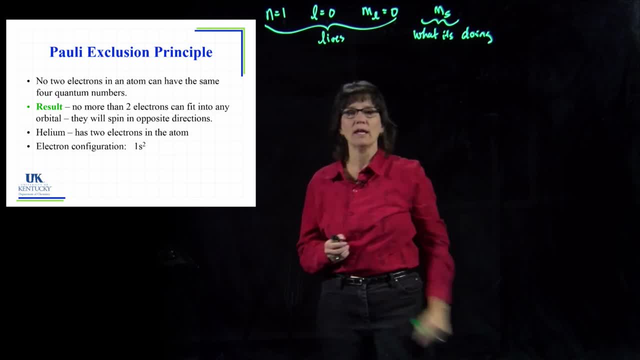 They are in the orbital that exists in a s subshell. It can have two electrons and we put that superscript two to show that it has two electrons in there And we can draw its orbital diagram. Its orbital diagram would show the orbital with a box. okay, 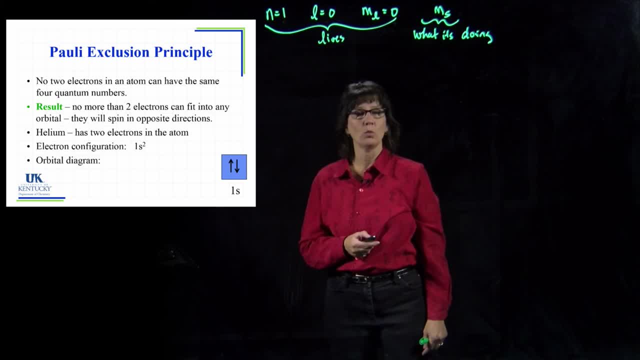 We name the subshell one s- That's the name of the orbital as well- And now this has two electrons, but they're spinning in opposite directions. When we do that, we could then also assign the quantum numbers for each one of those electrons. 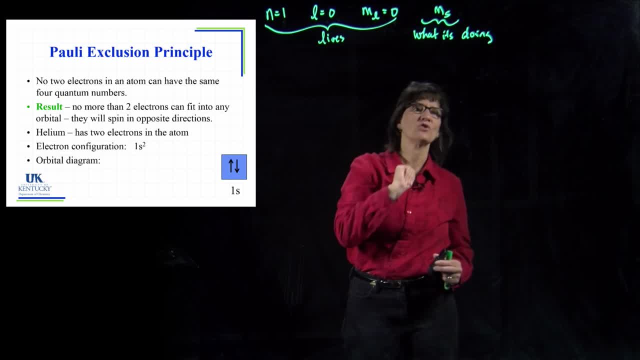 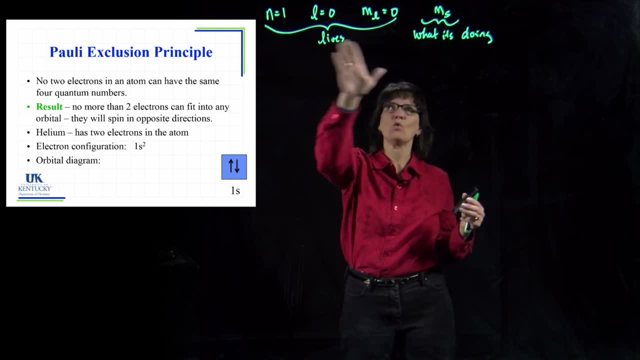 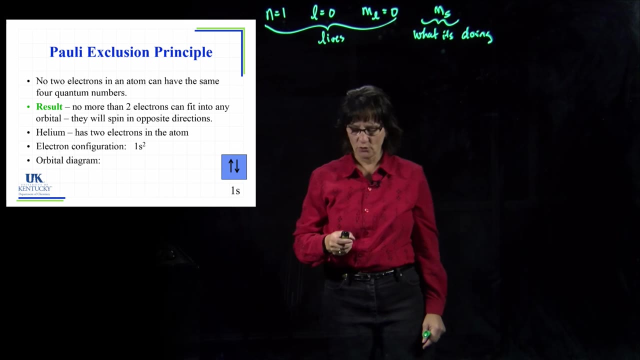 So each electron will have four quantum numbers associated with it. I don't care if that atom has 23 electrons in it. Every electron in it will have a set of quantum numbers that tell where that electron lives and what that electron is doing. So let's give the quantum numbers for these two electrons. 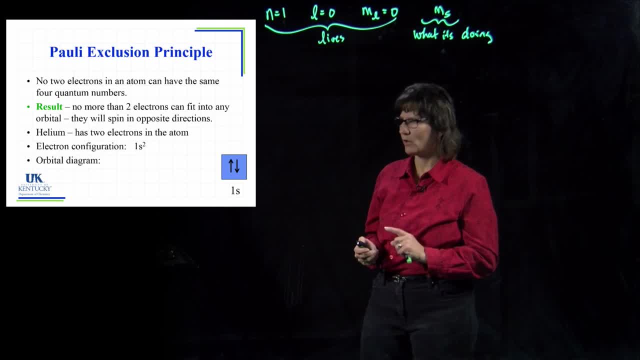 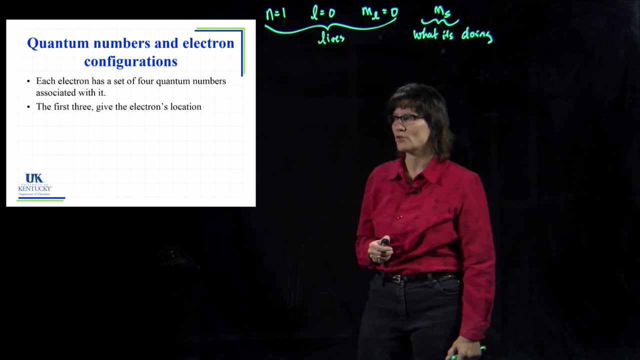 Where does it live and what is it doing? Oh no, we're not going to do that yet. We'll do that in a minute. Alright, That's what I just said. Each electron has a set of four quantum numbers associated with it.